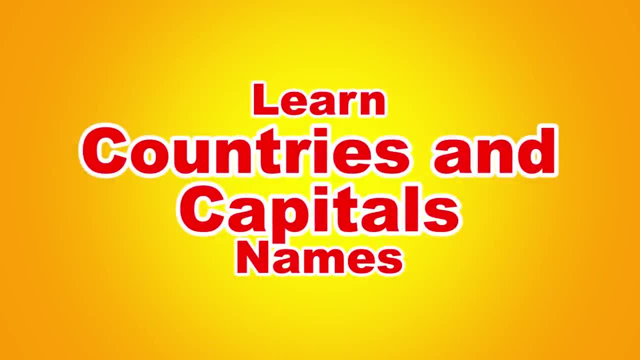 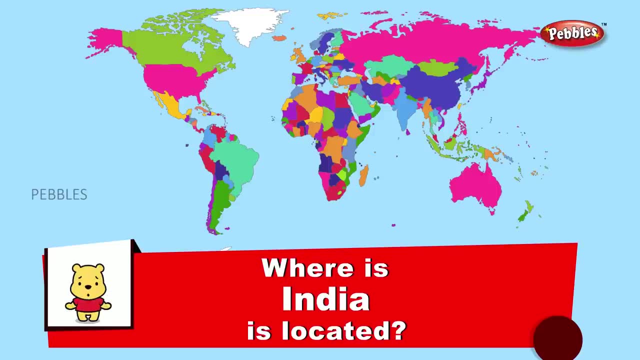 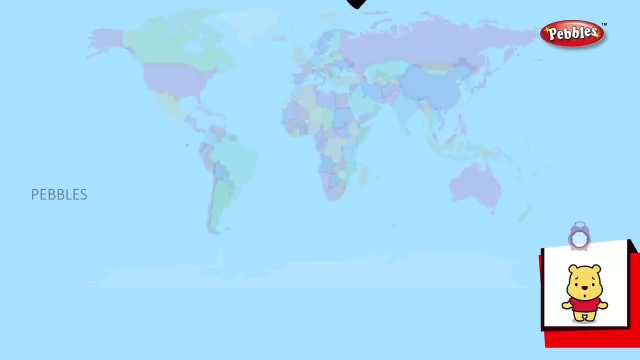 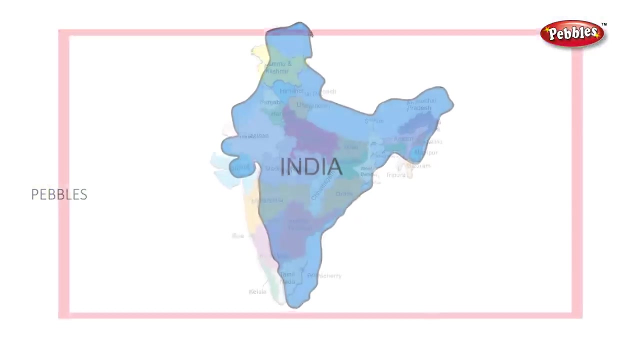 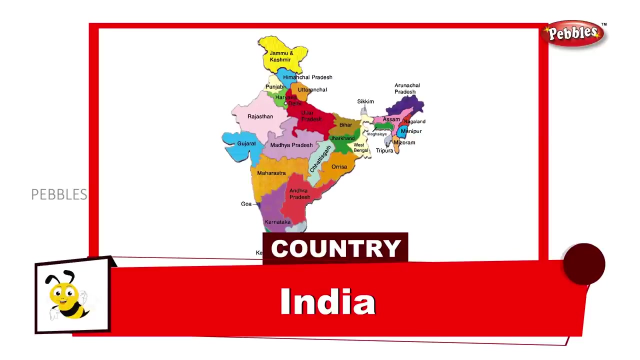 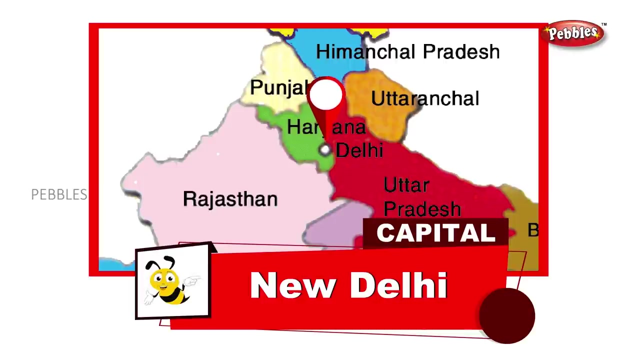 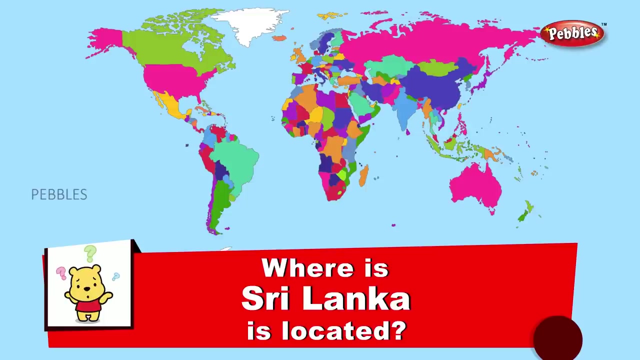 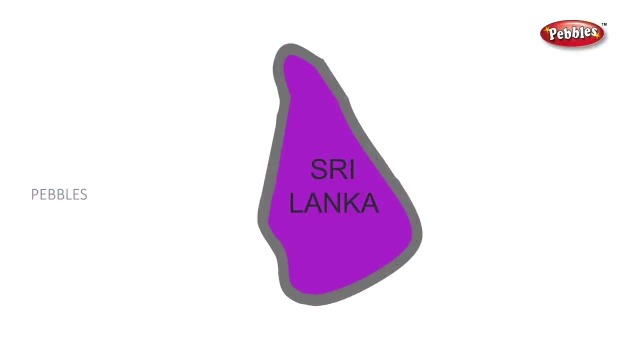 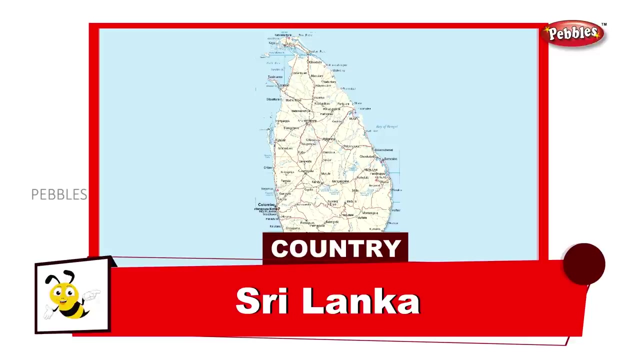 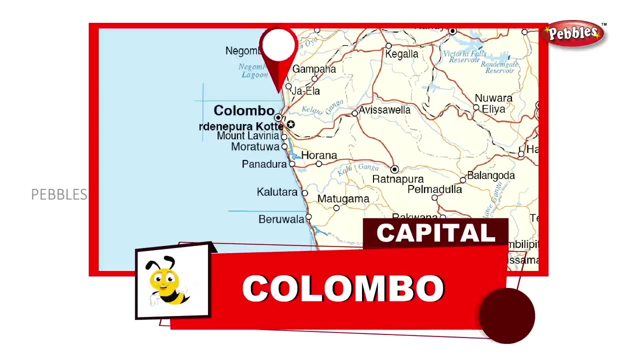 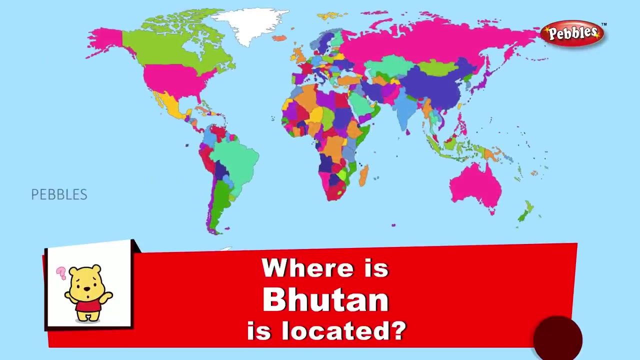 Learn countries and capitals names. Where is India located? It's here, Country India Capital, New Delhi. Where is Sri Lanka located? It's here, Country Sri Lanka Capital, Colombo. Where is Bhutan located? It's here. 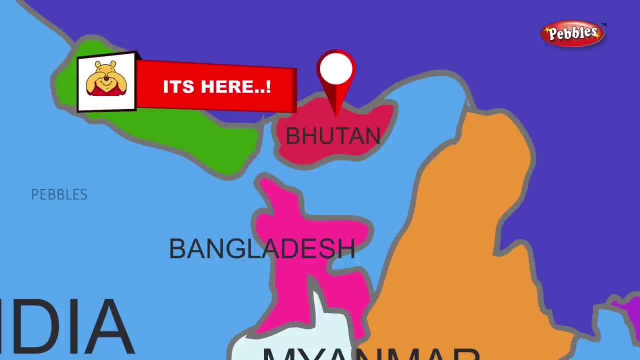 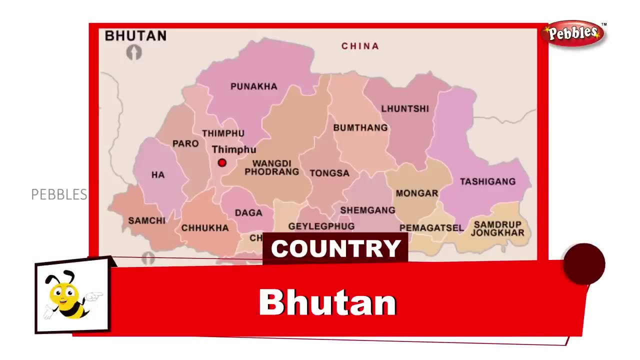 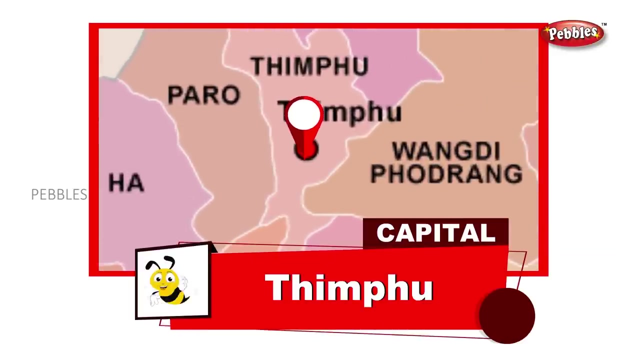 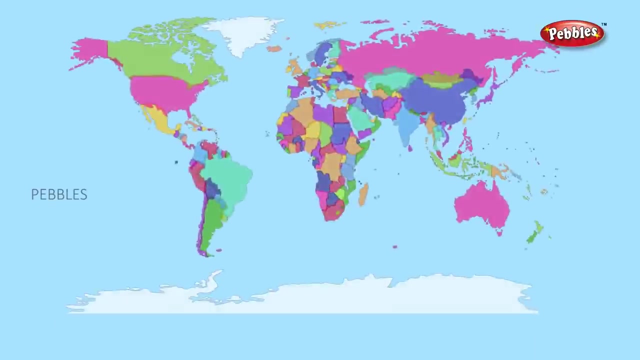 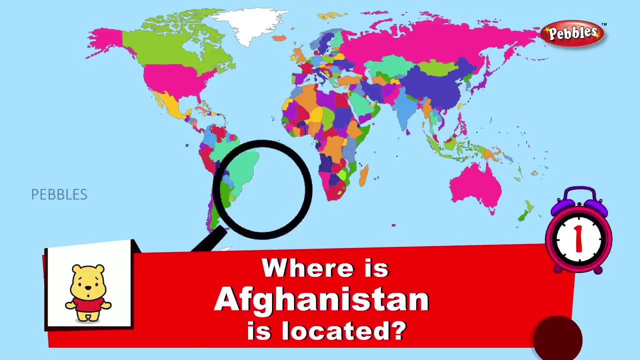 Country Bhutan, Capital Thimphu. Where is India located? It's here, Country Bhutan, Capital Thimphu. Where is India located? It's here, Capital Thimphu. Where is India located. 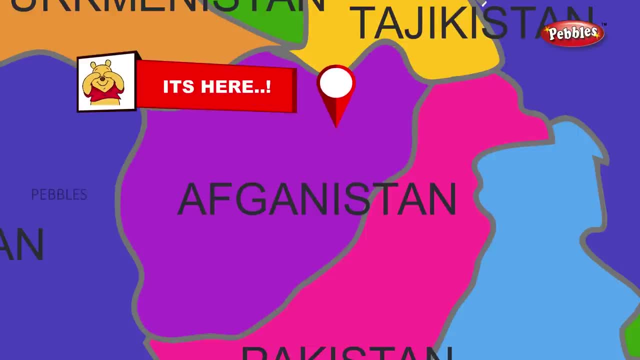 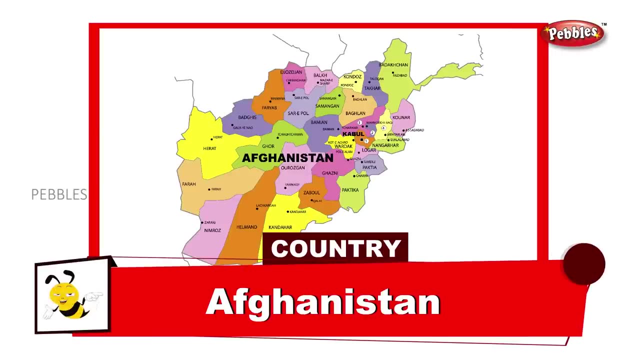 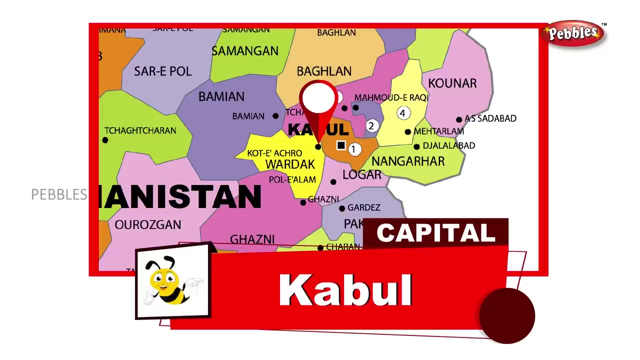 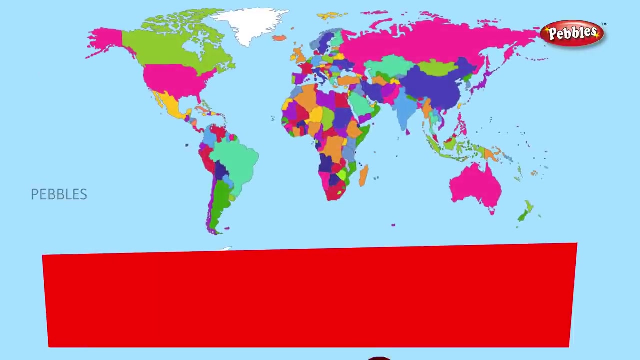 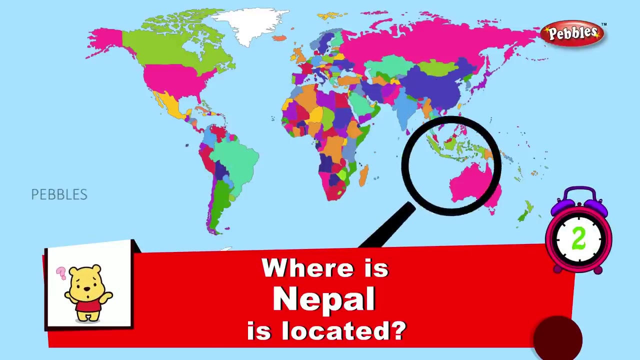 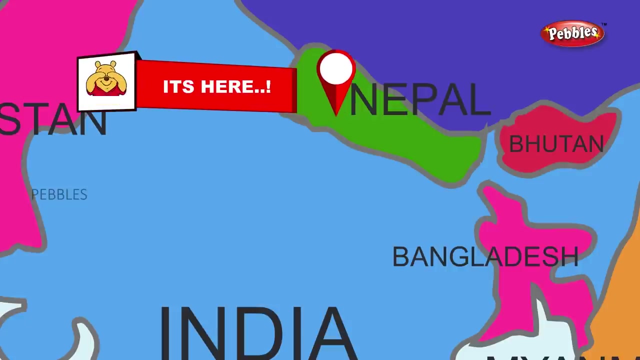 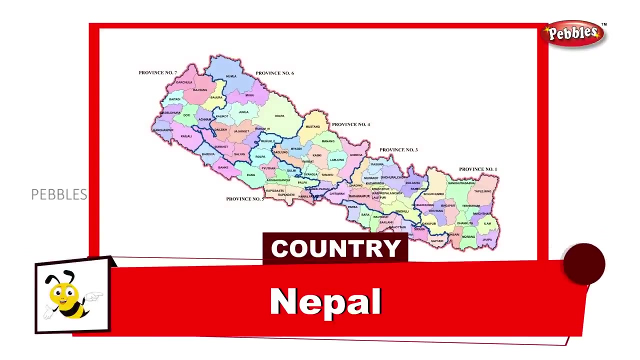 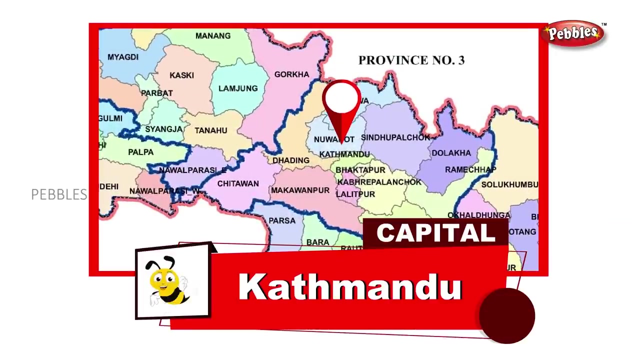 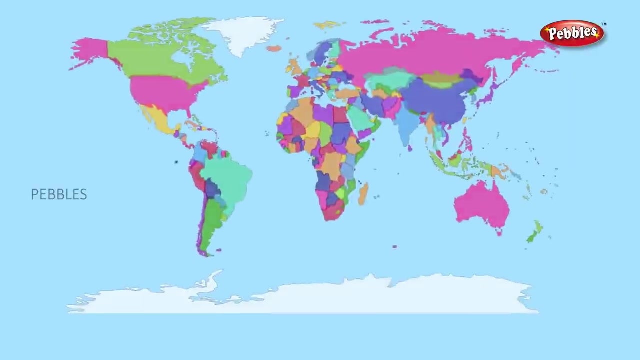 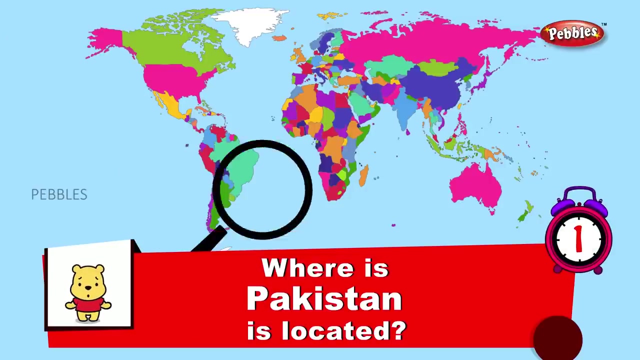 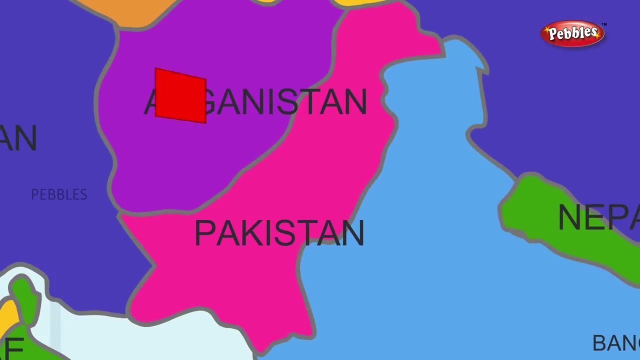 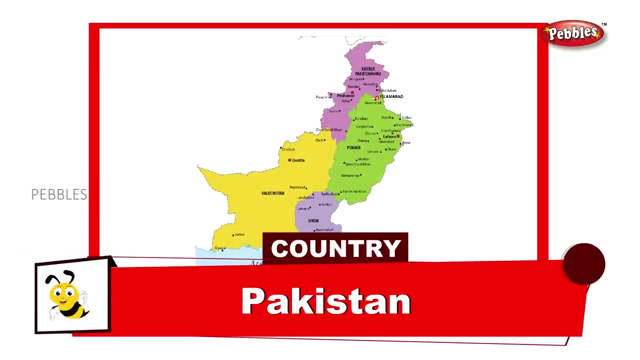 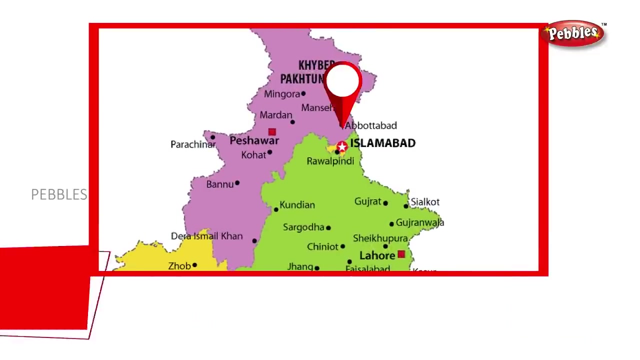 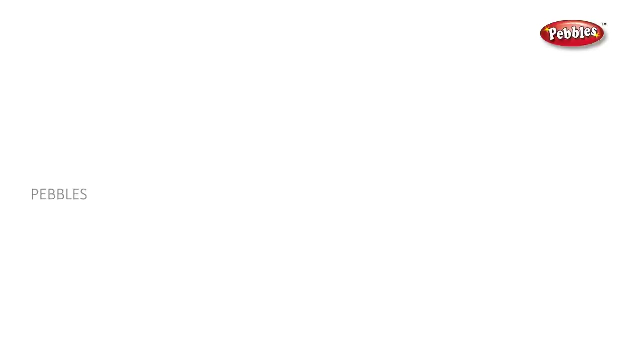 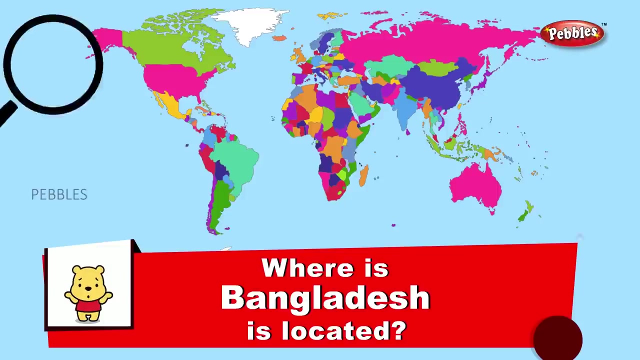 It's here, Country India, Capital, Thimphu. Country, India. Where is Nepal located? It's here, Nepal, Kathmandu. Where is Pakistan located? It's here, Pakistan, Islamabad. Where is Bangladesh located? 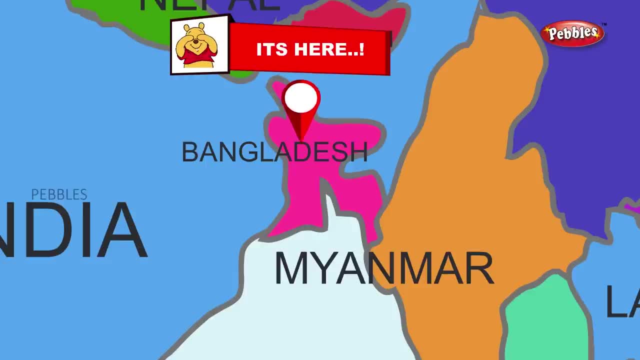 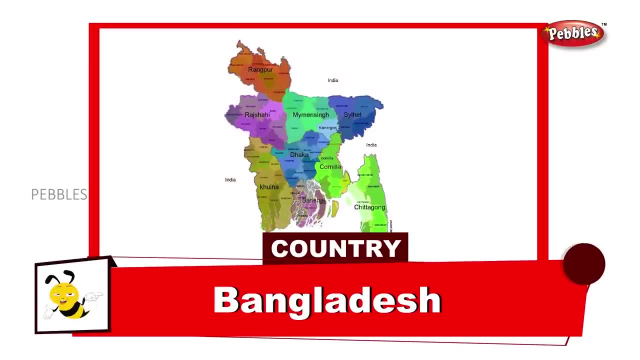 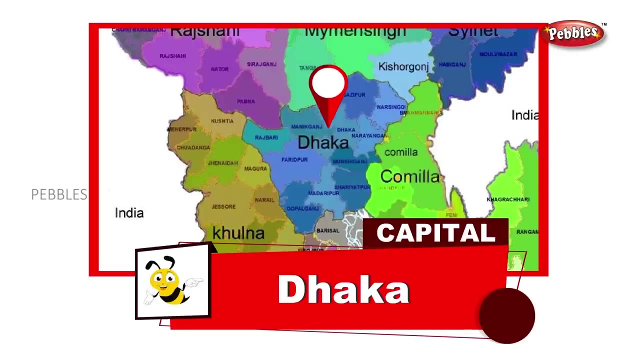 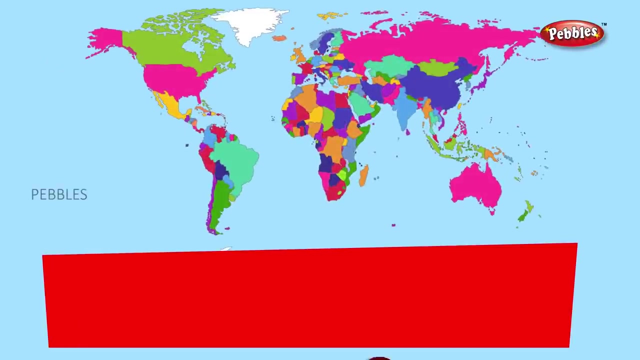 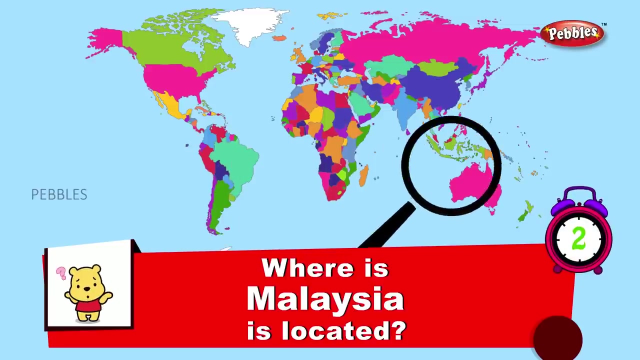 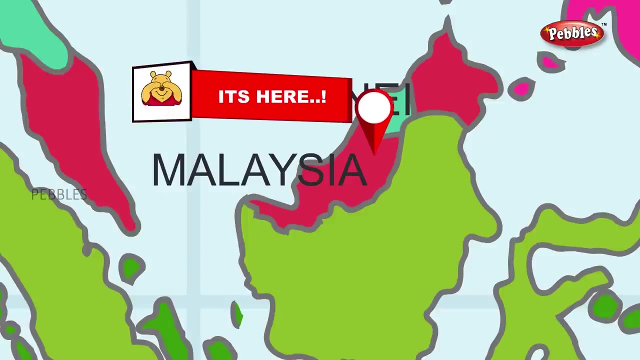 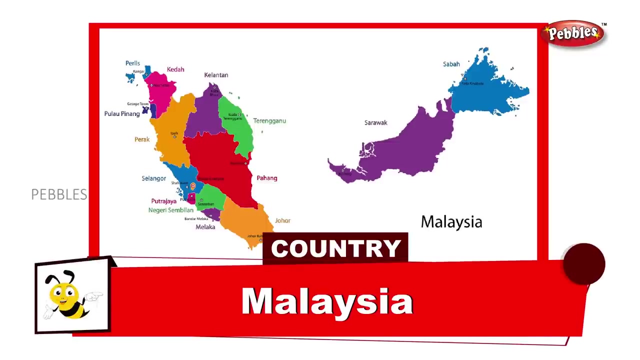 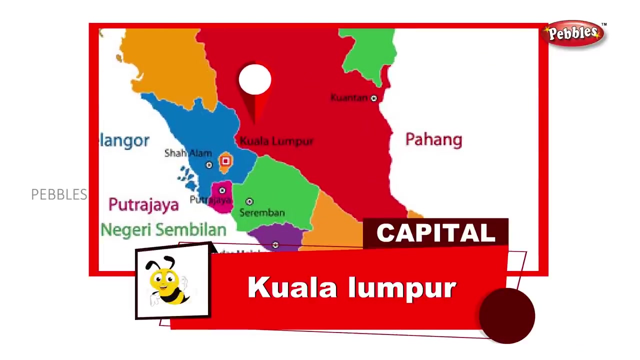 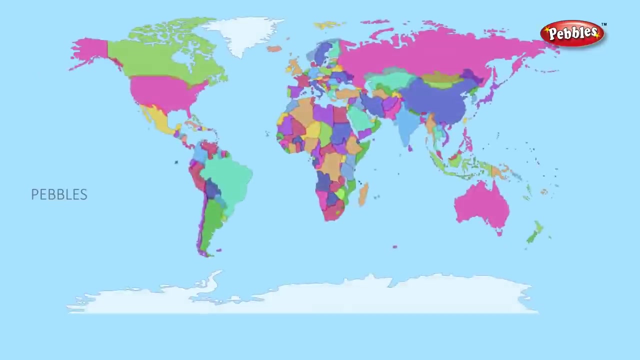 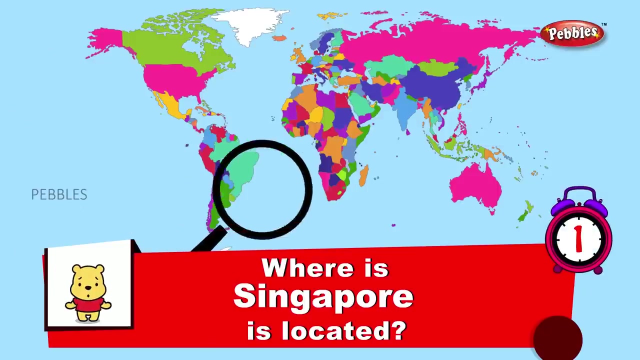 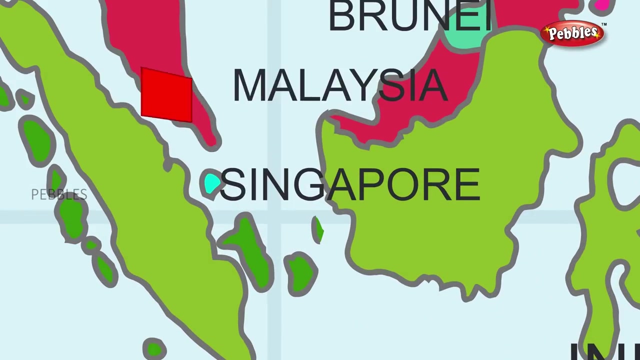 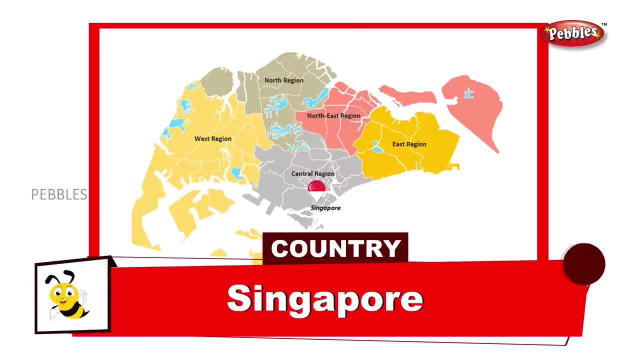 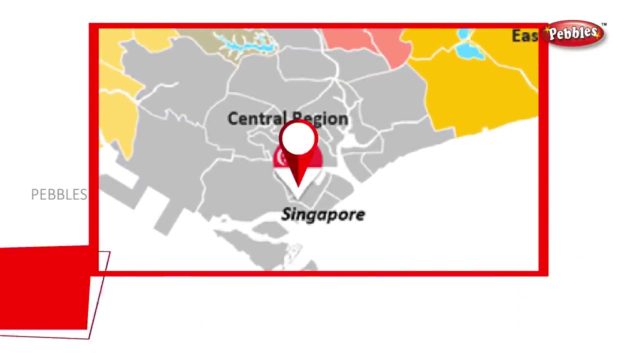 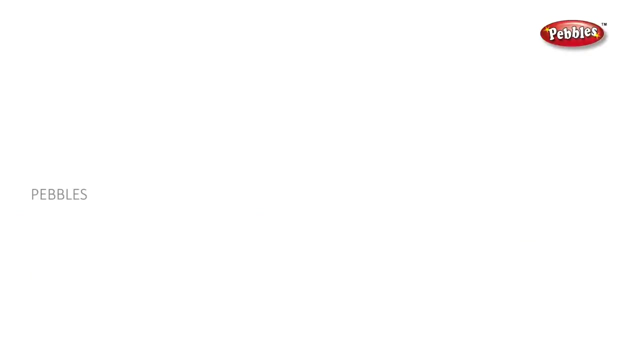 It's here, Bangladesh, Dhaka, Kuala Lumpur. It's here, Country Malaysia, Capital, Kuala Lumpur. Where is Singapore located? It's here. It's here, Country, Singapore, Capital, Singapore. Where is Thailand located? 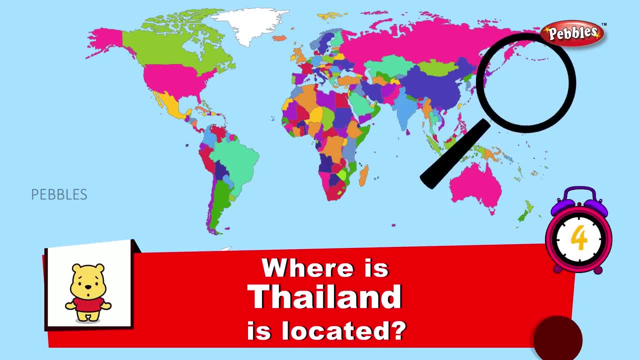 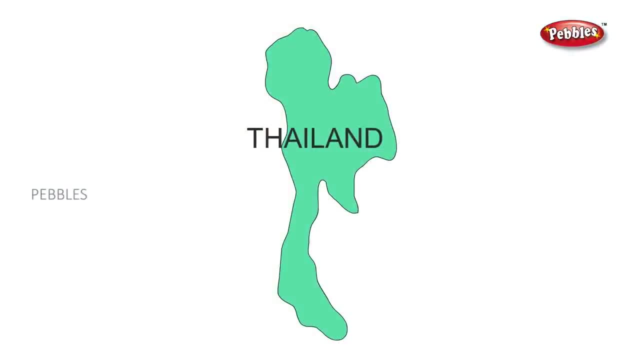 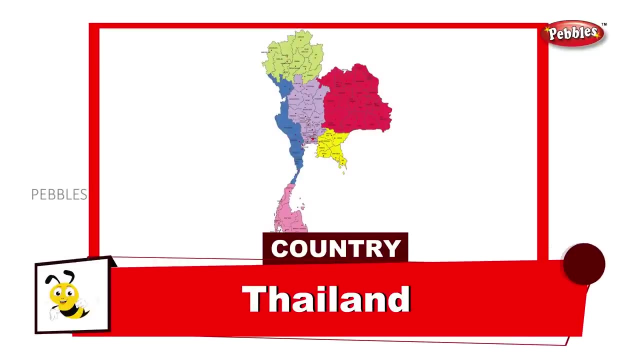 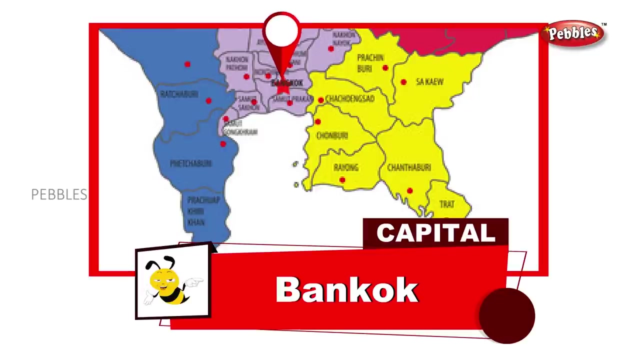 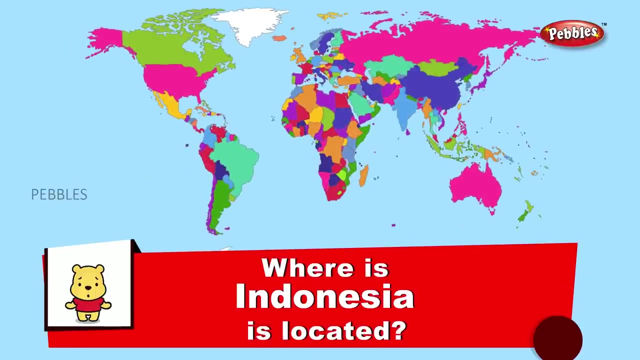 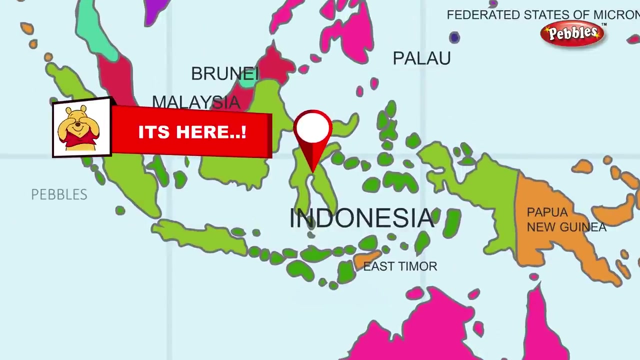 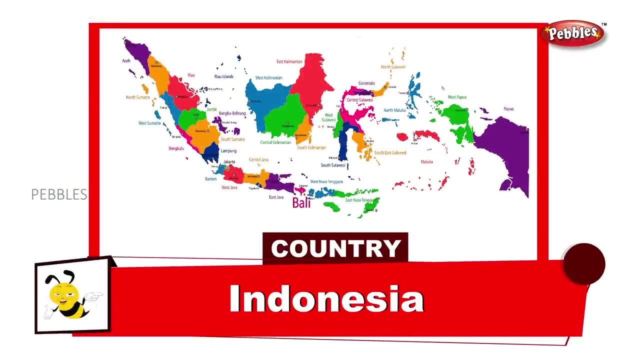 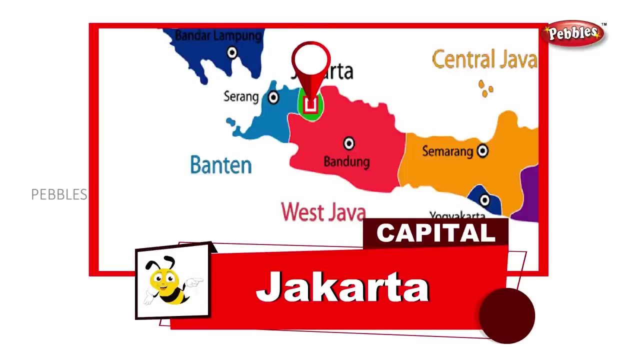 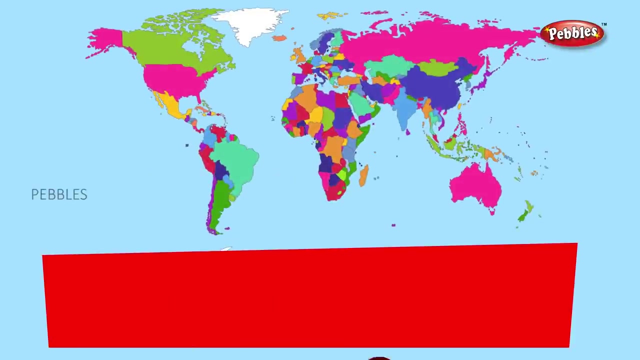 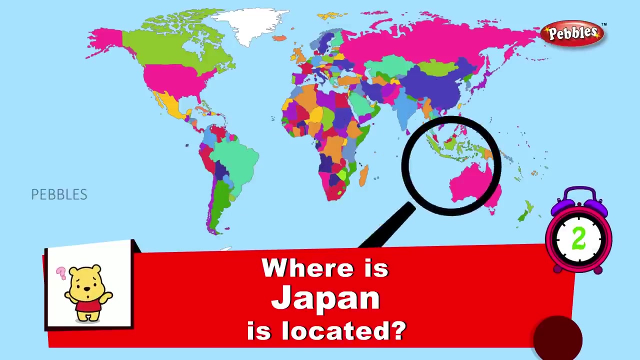 It's here, Thailand. It's here. Country Thailand, Capital Bangkok. Where is Indonesia located? It's here. It's here. Country Indonesia: Capital Jakarta. Where is Japan located? Where is Japan located? It's here, Japan. 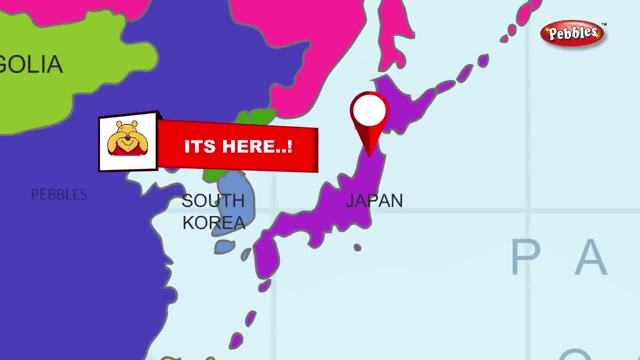 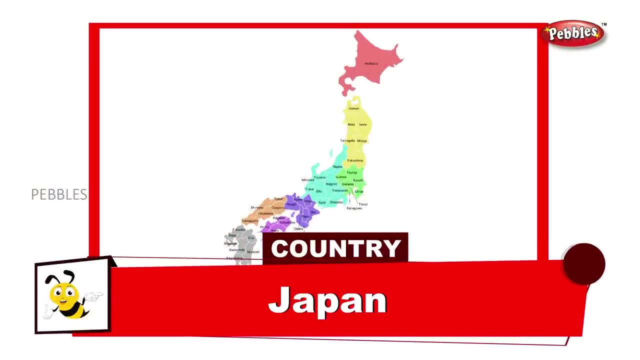 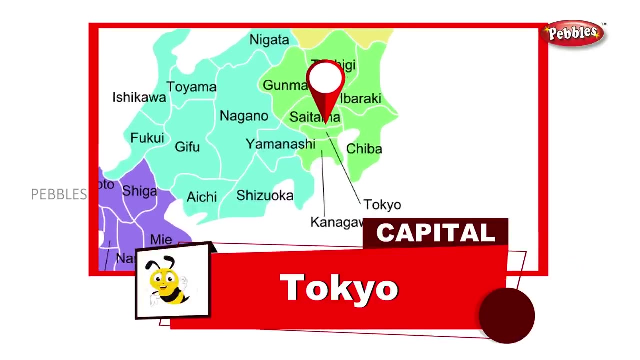 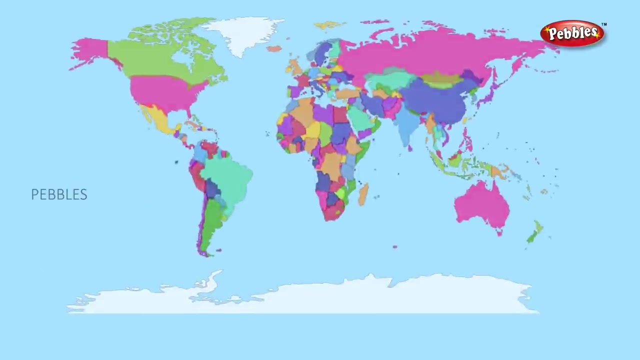 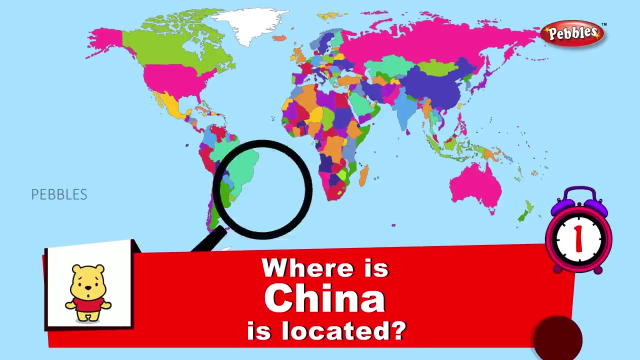 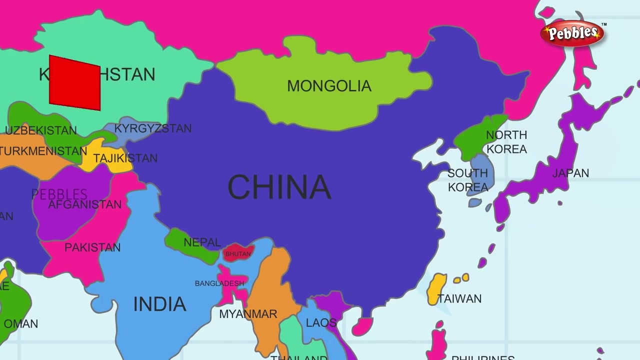 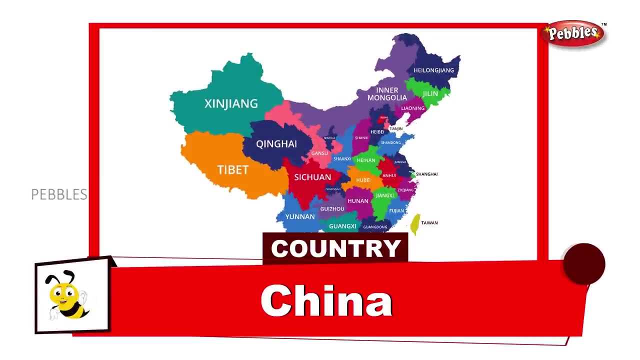 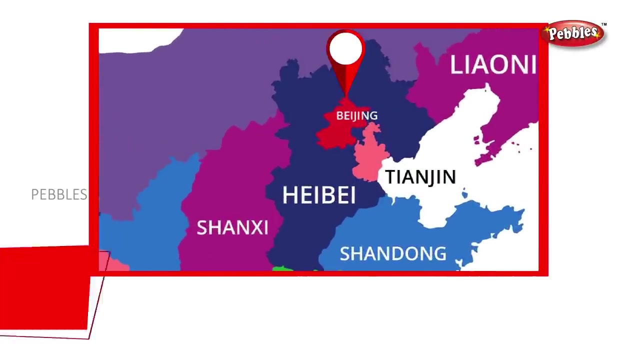 China, India, Singapore. It's here Congress, China, Japan. It's here TOKYO, Singapore, China, Japan, Japan territory. It's here Japan. Where is China located? It's here Country China. 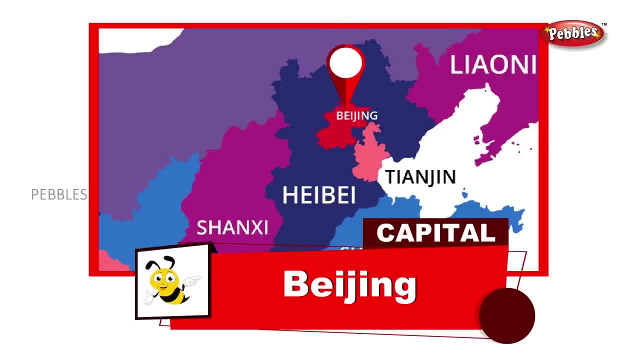 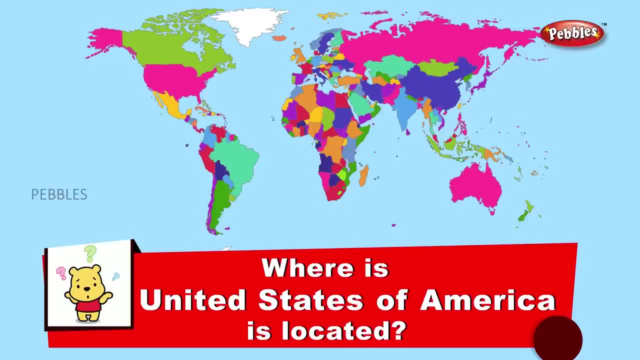 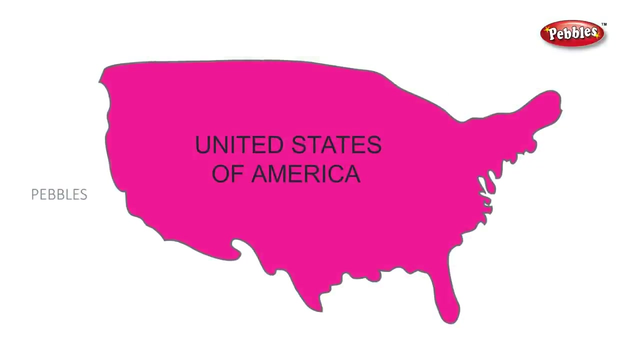 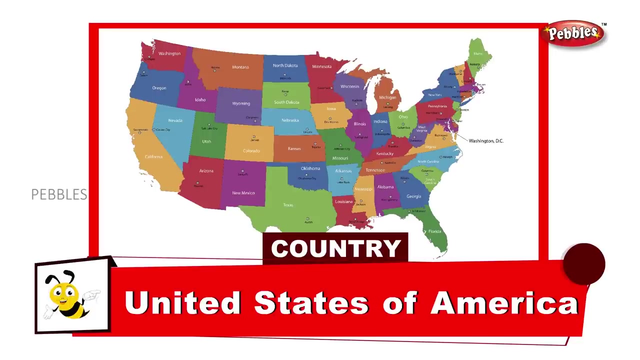 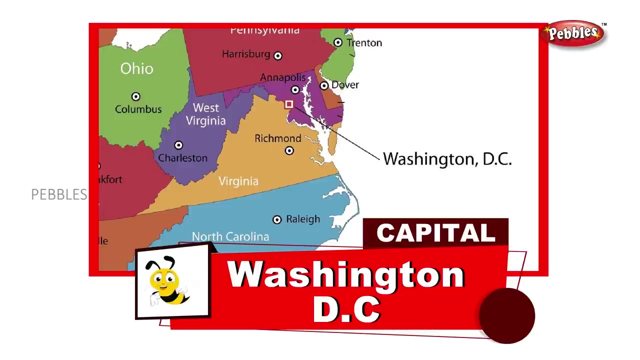 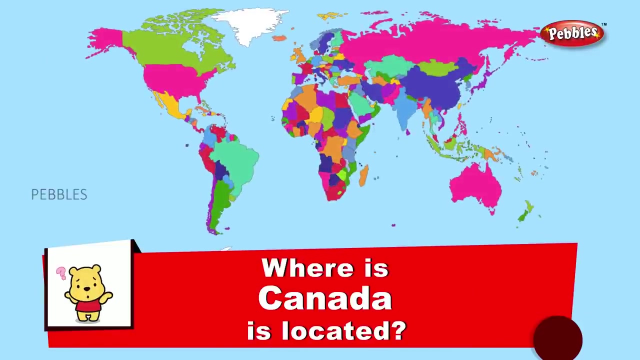 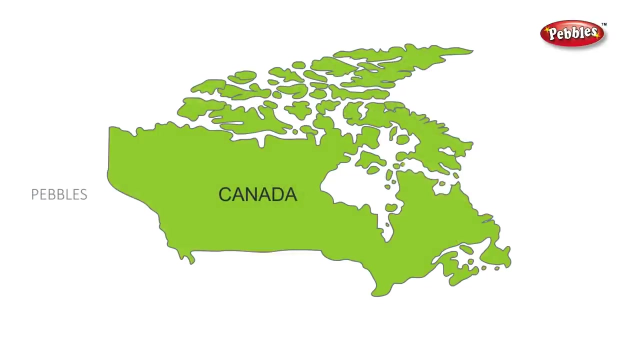 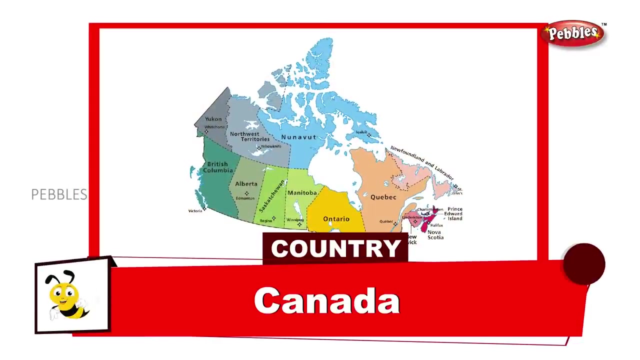 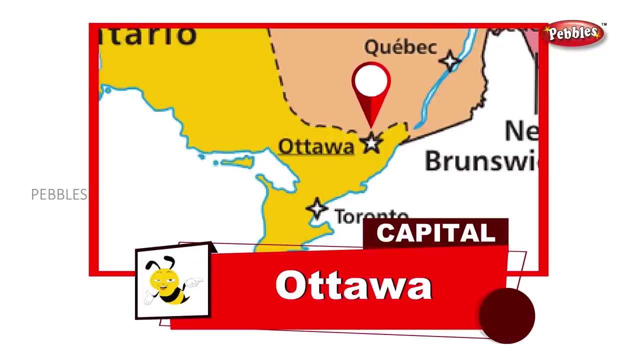 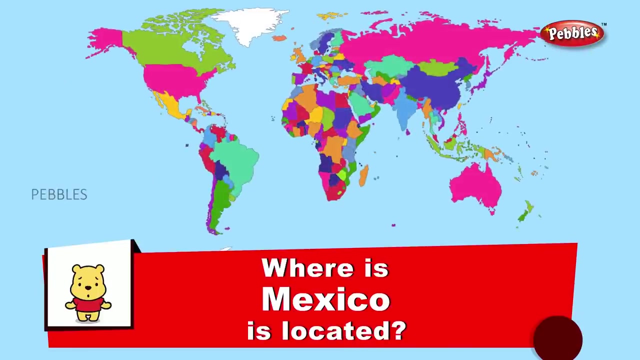 Capital, Beijing. Where is United States of America is located? It's here, Country, United States of America Capital, Washington DC. Where is Canada located? It's here, Country, Canada Capital, Ottawa. Where is Mexico located? 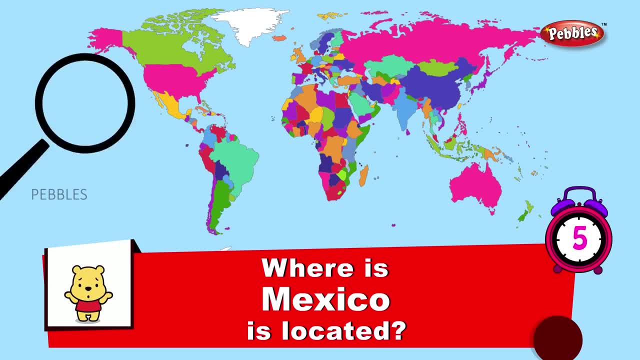 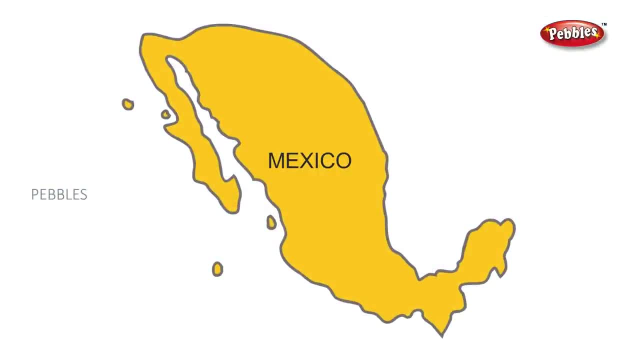 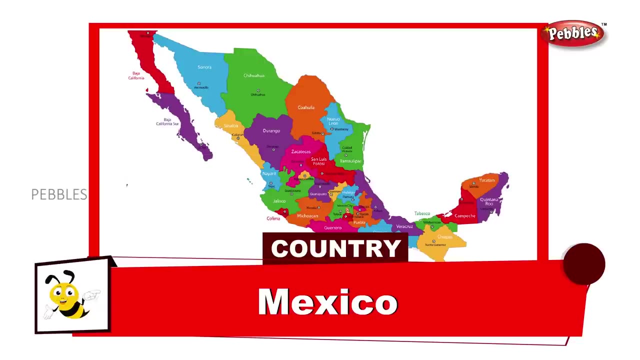 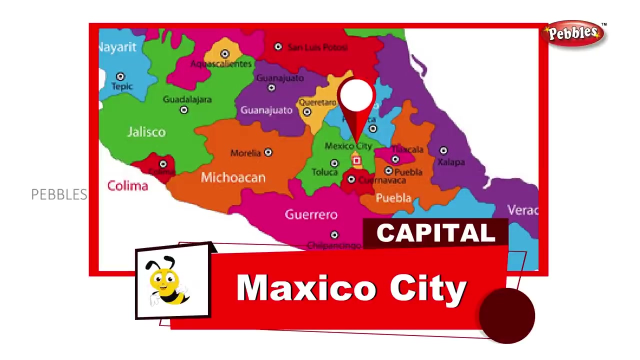 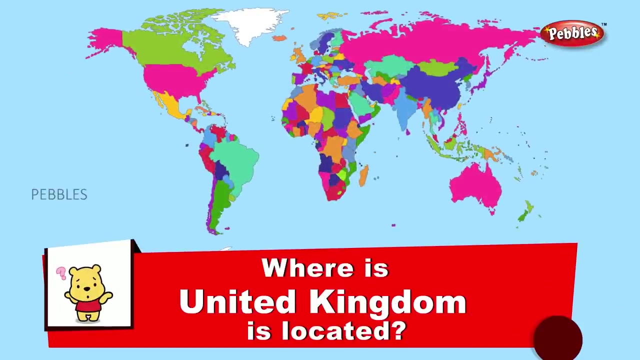 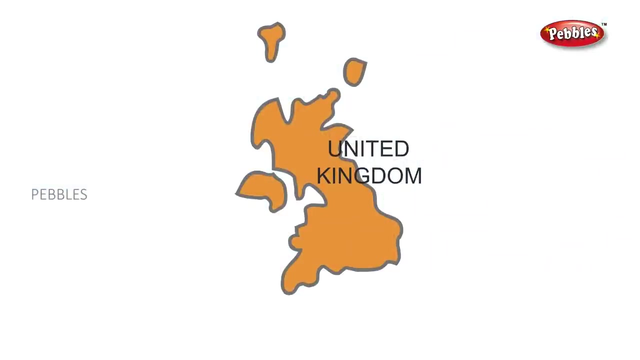 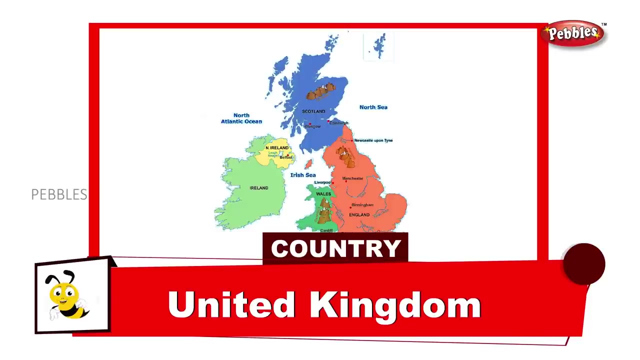 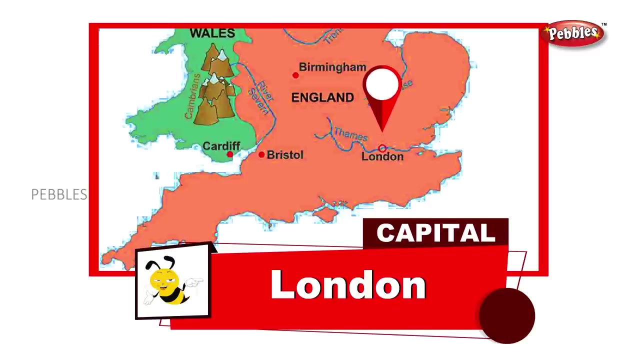 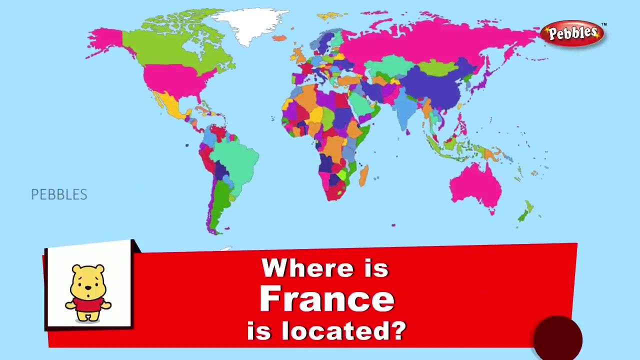 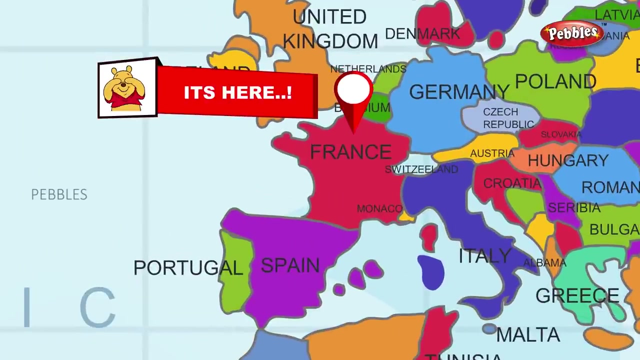 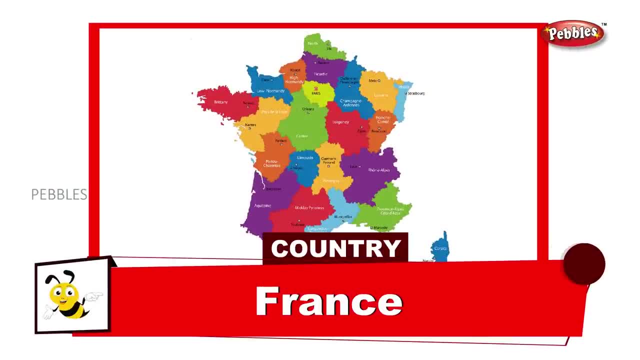 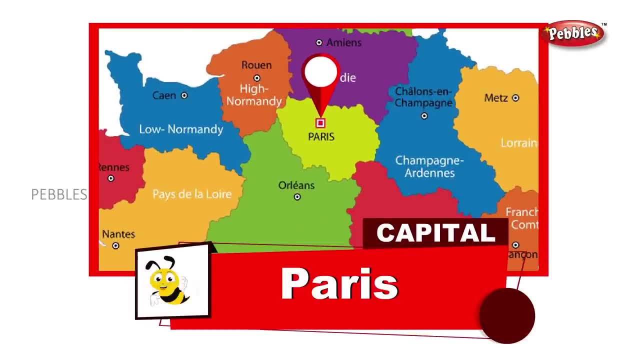 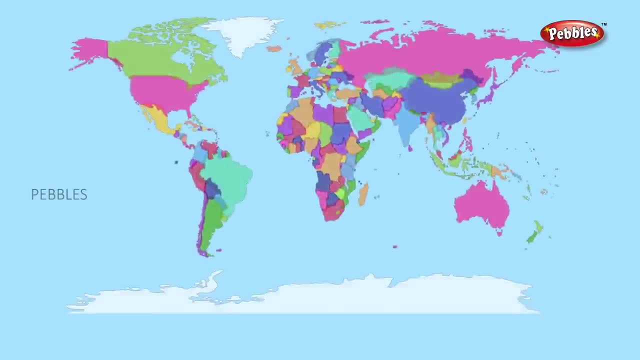 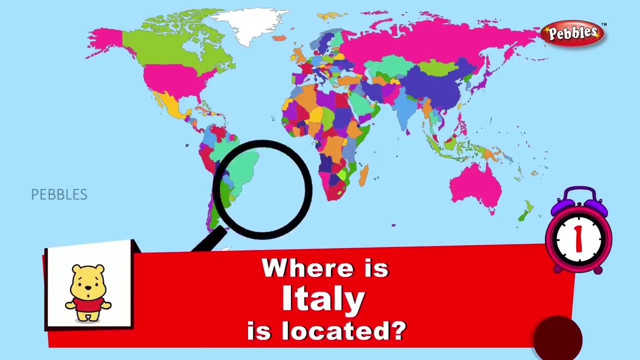 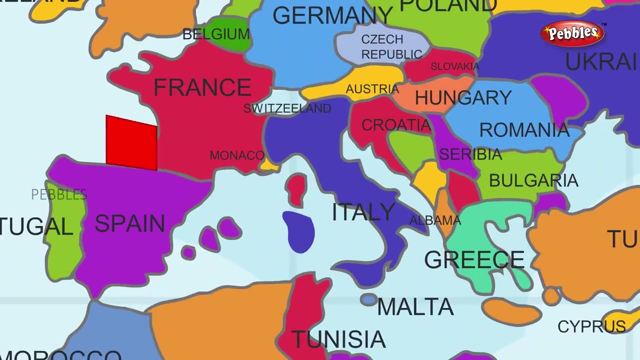 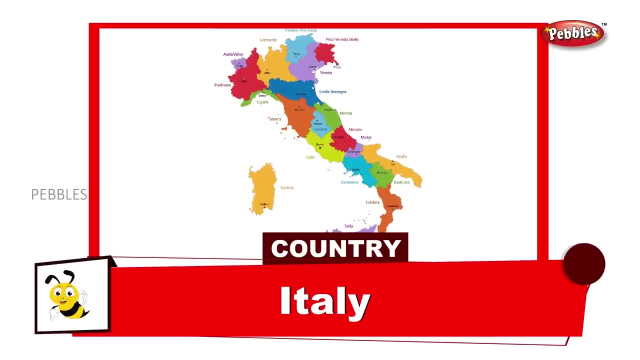 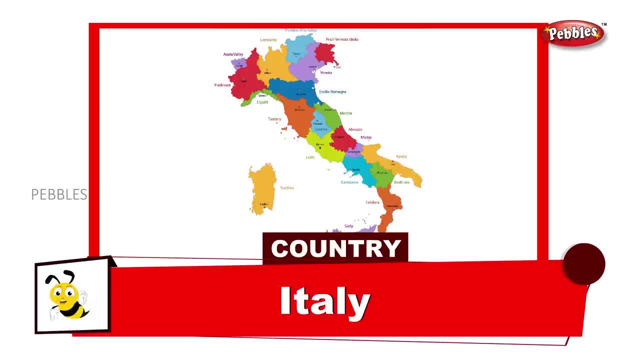 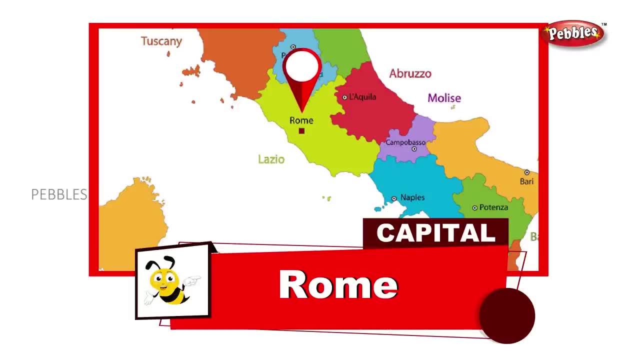 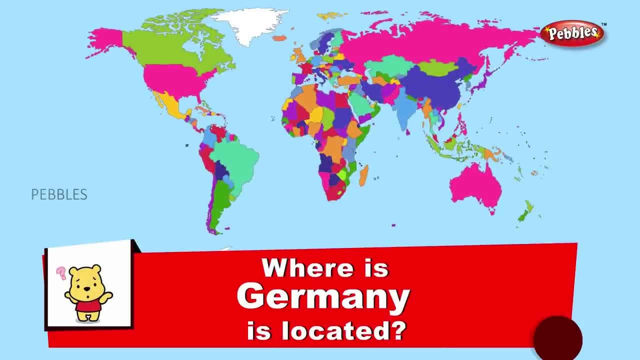 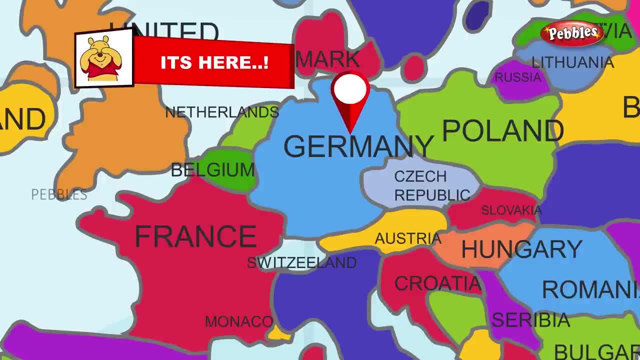 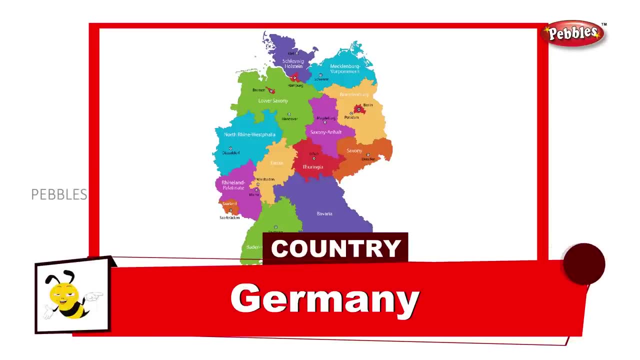 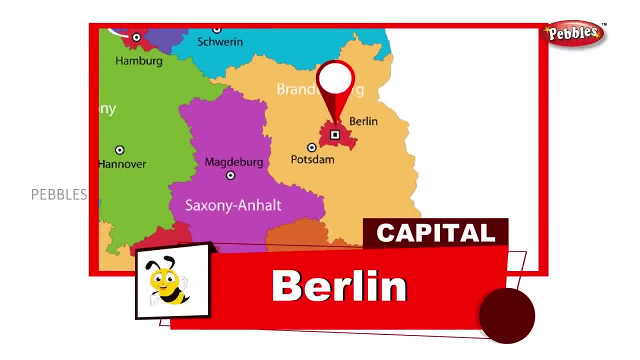 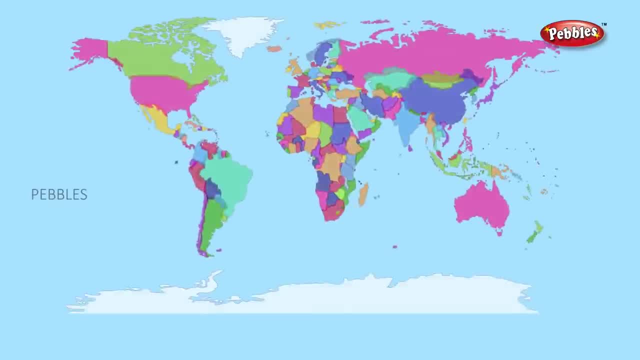 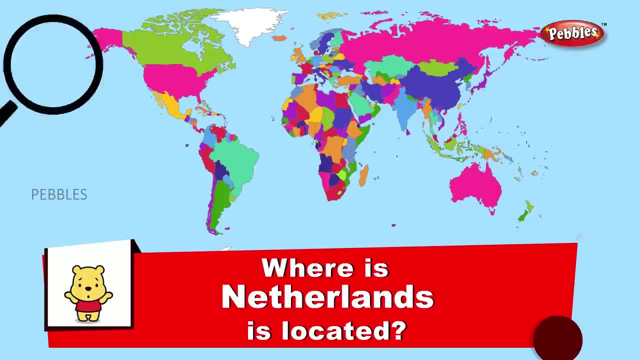 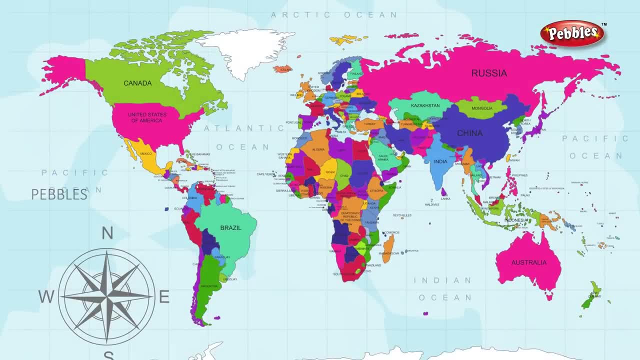 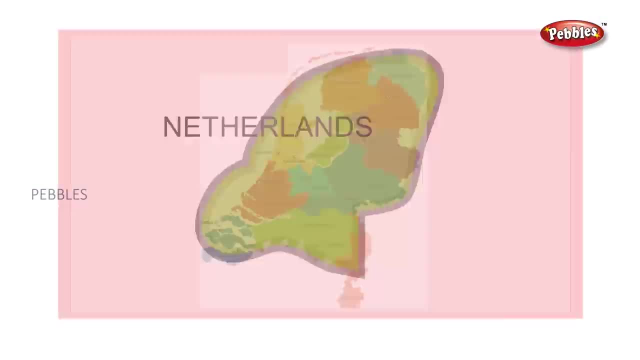 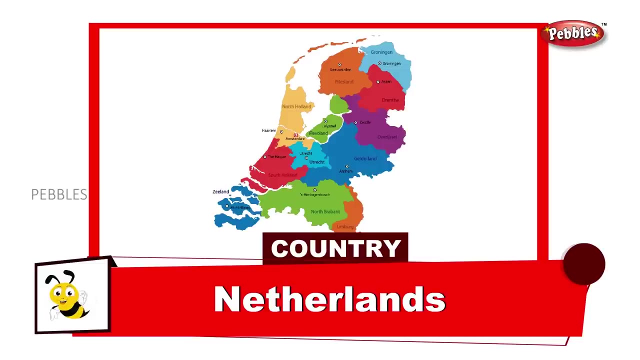 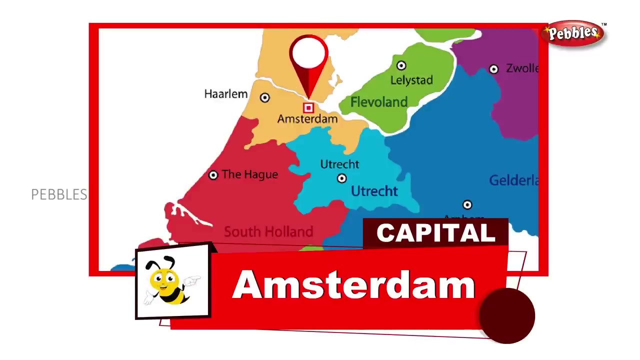 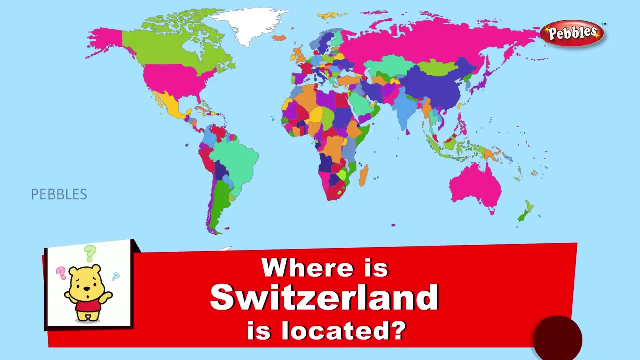 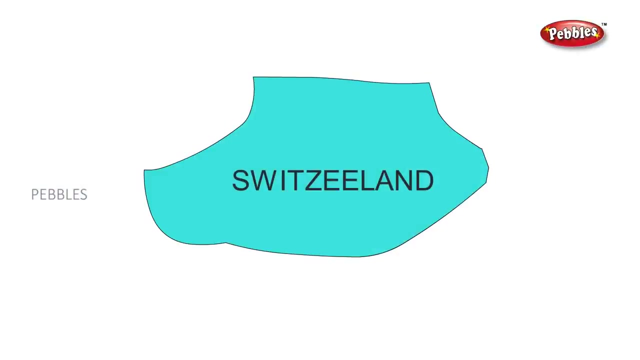 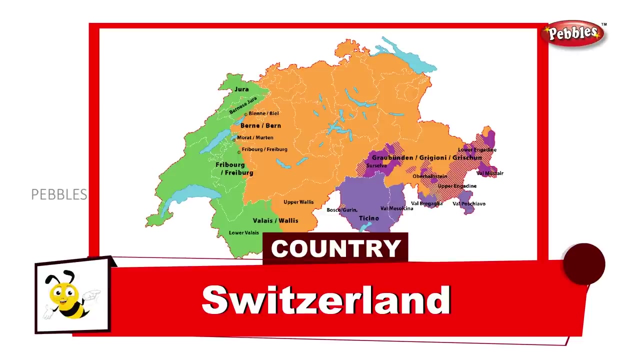 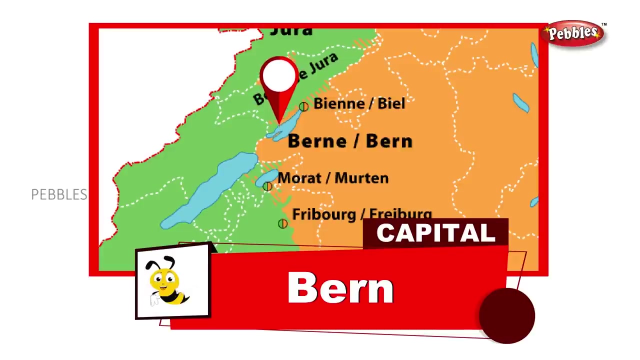 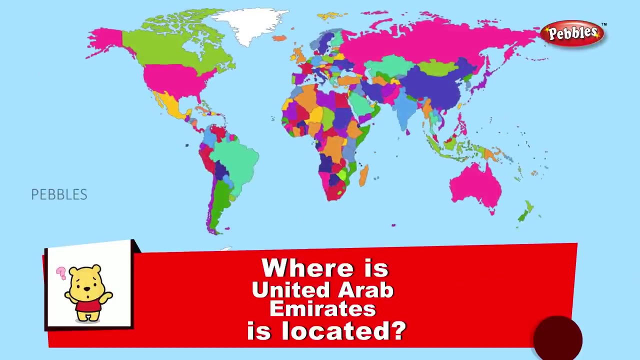 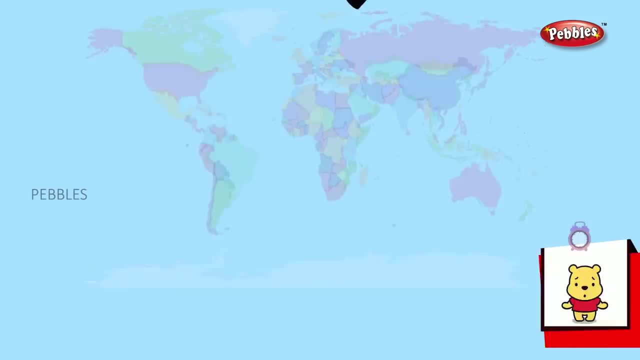 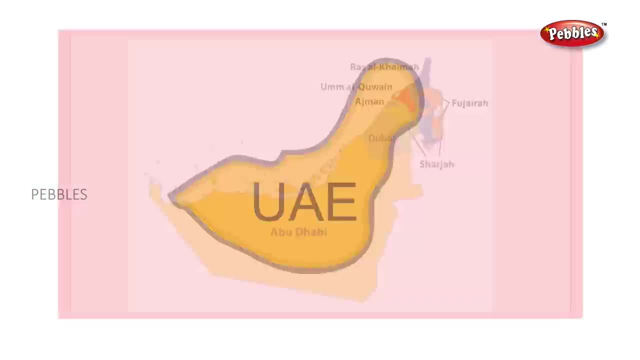 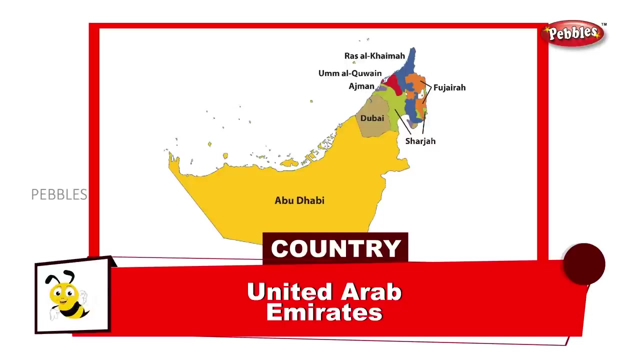 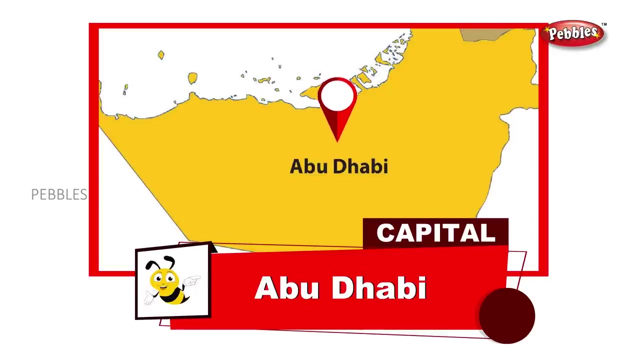 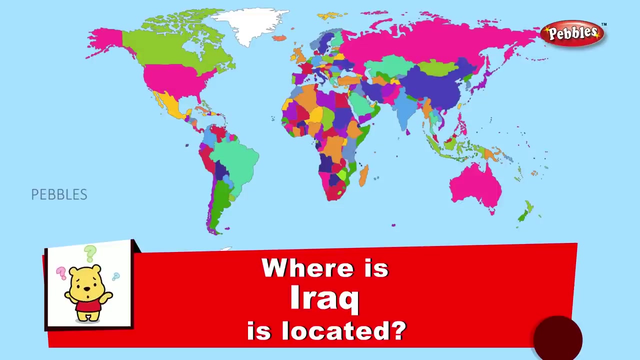 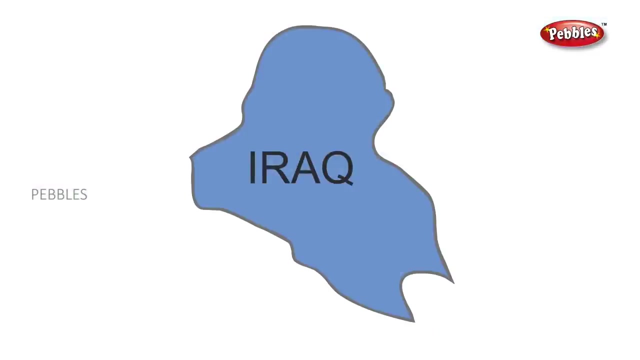 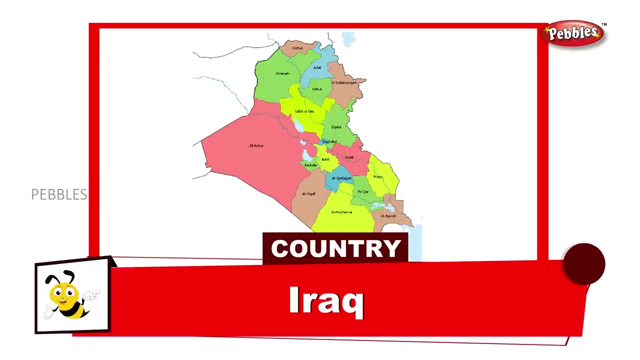 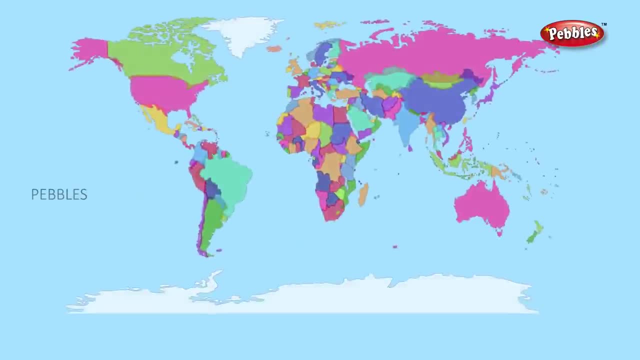 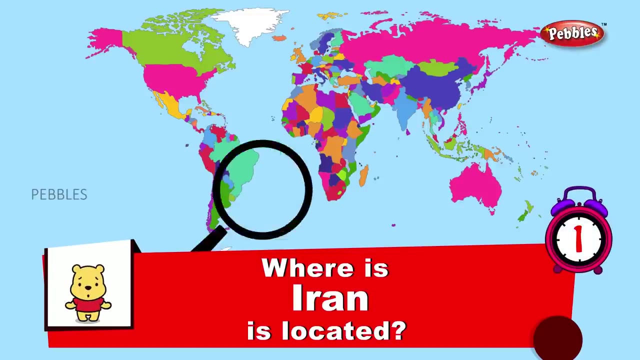 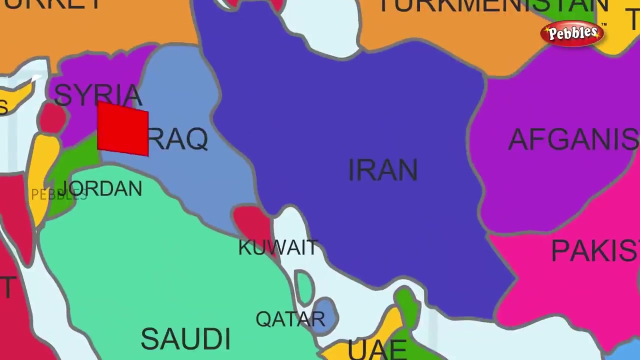 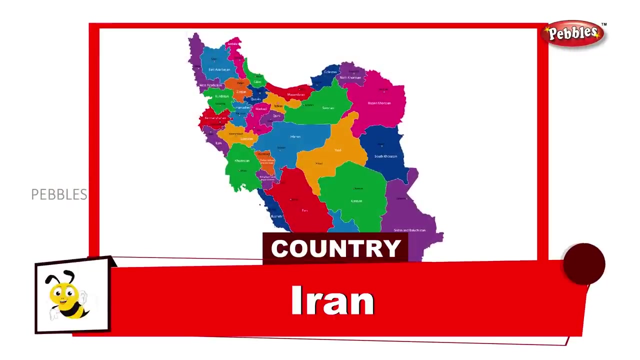 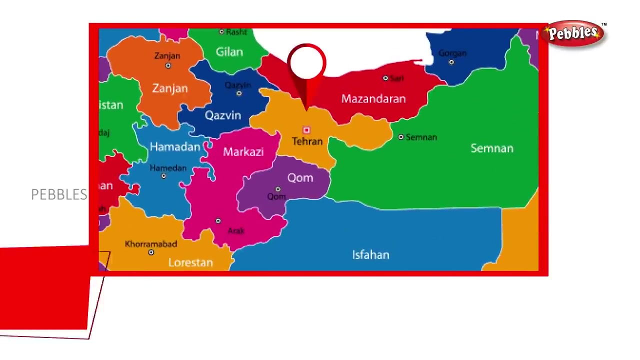 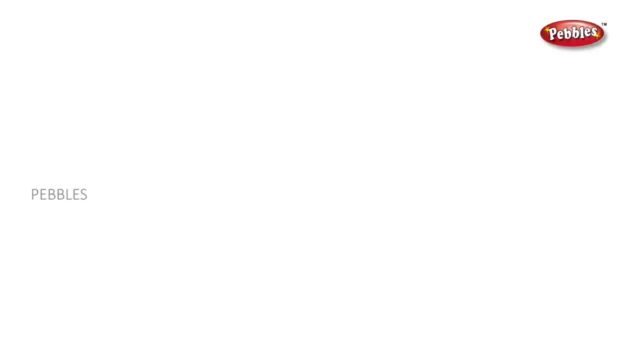 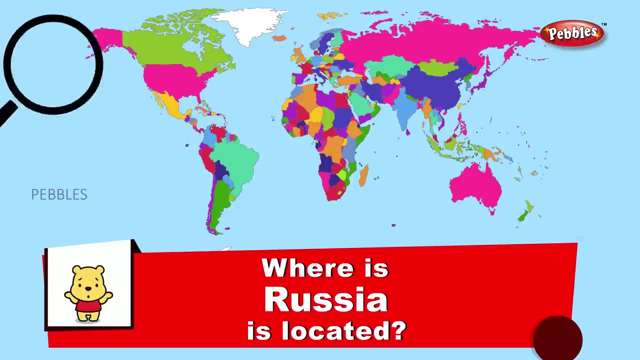 It's here, Where is Iran located? It's here, Country Country. It's here, Country Country. It's here Country Country, Iran. Iran, Capital, Iran. Where is Russia located? It's here, Where is Russia located. 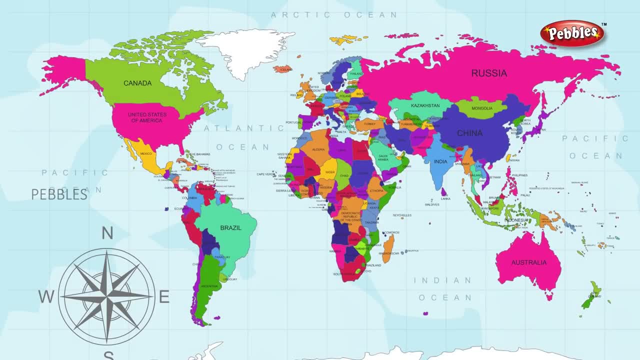 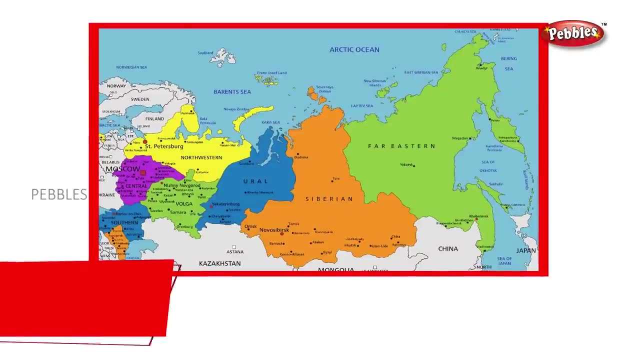 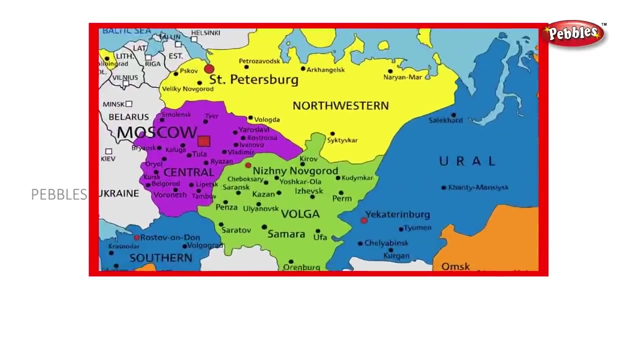 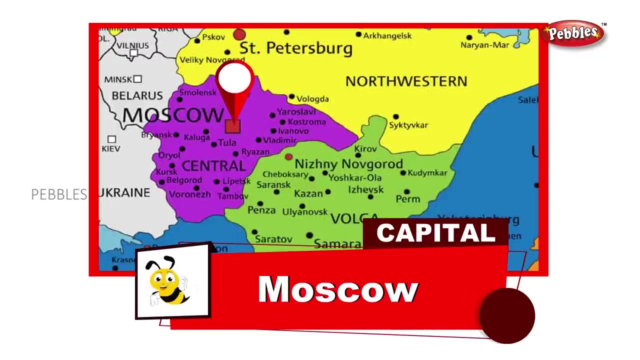 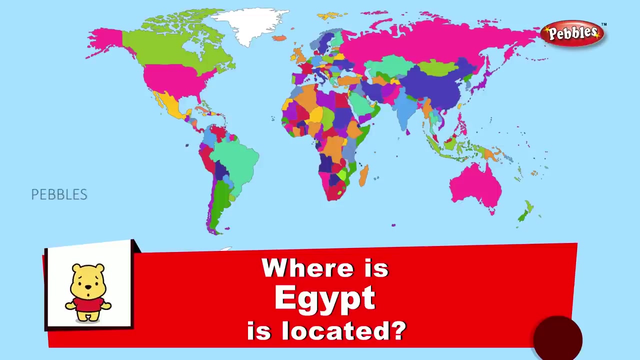 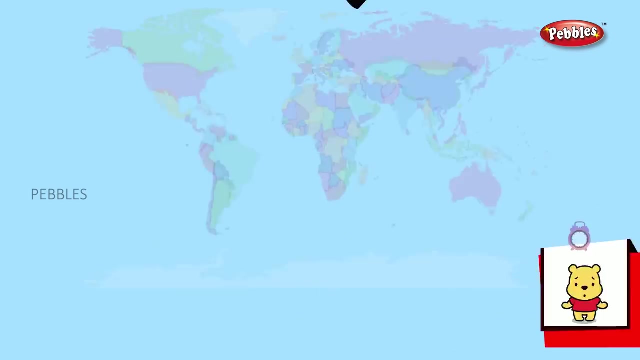 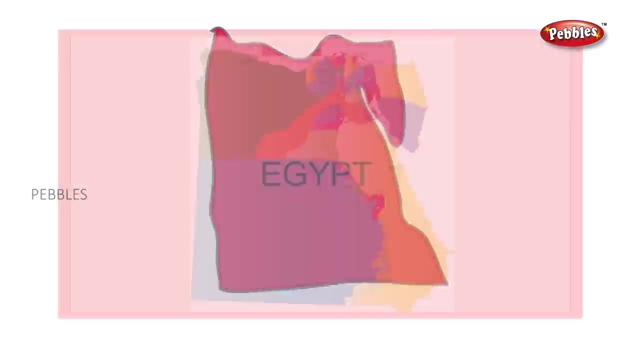 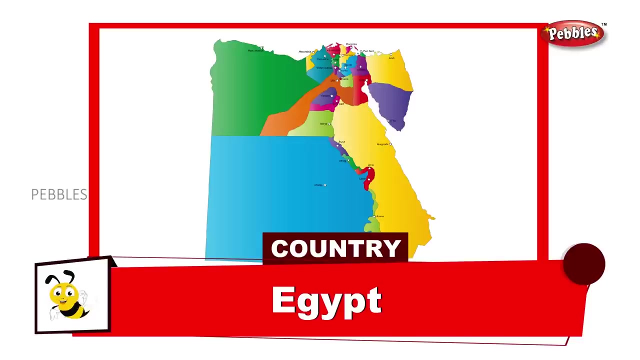 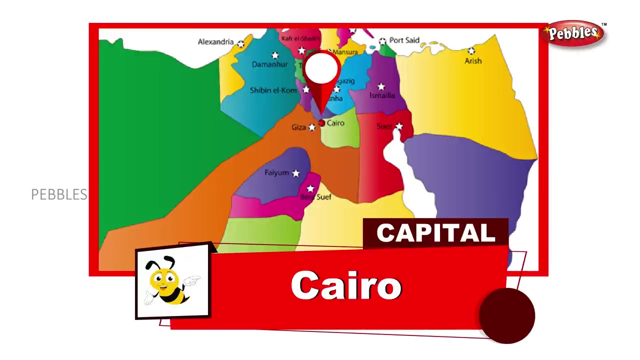 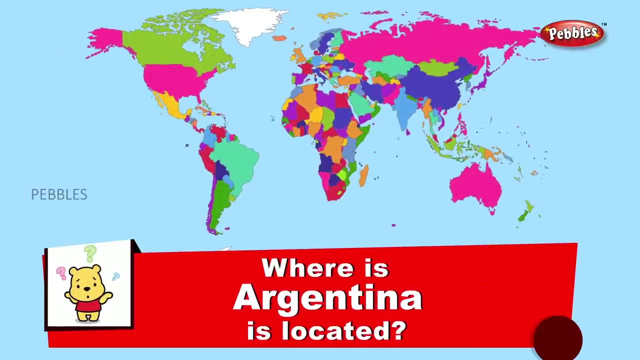 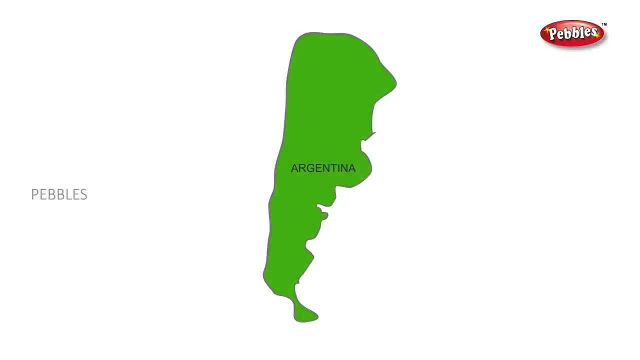 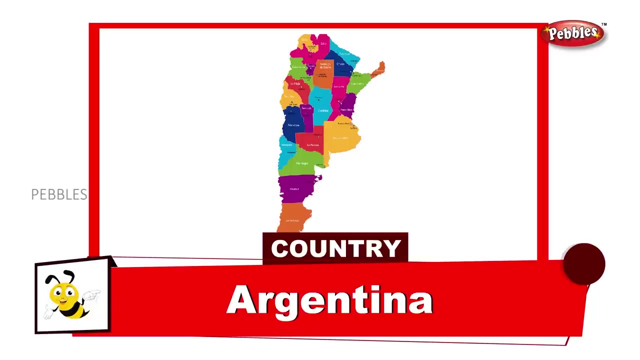 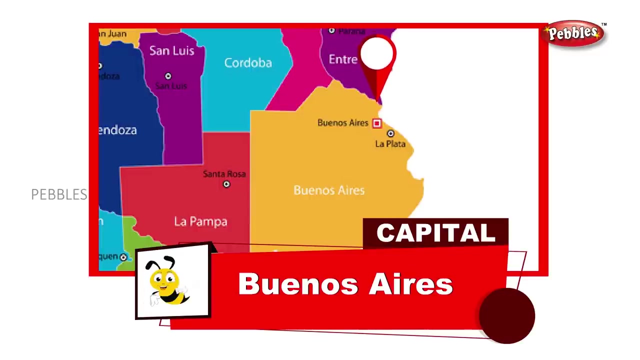 It's here. It's here, Country Russia, Capital Moscow. Where is Egypt located? It's here, Country Egypt, Capital Cairo. Where is Argentina located? It's here, Country Argentina. Country Argentina, Capital Buenos Aires. 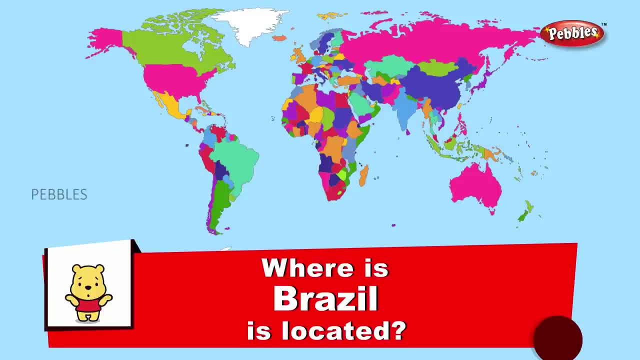 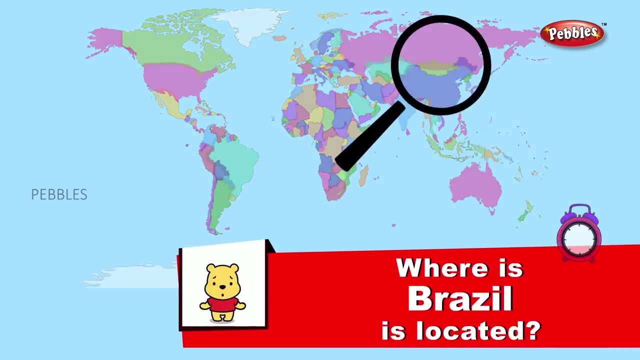 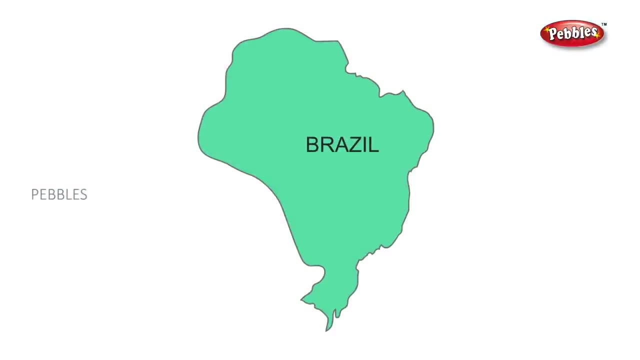 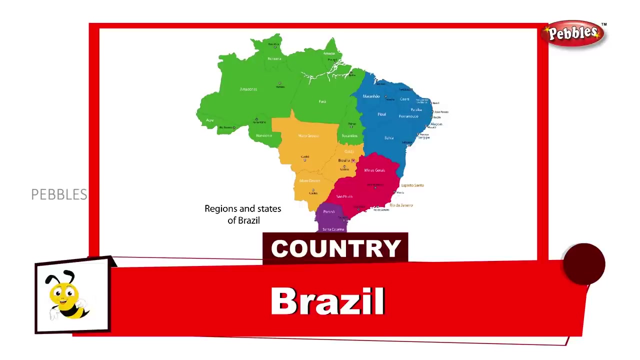 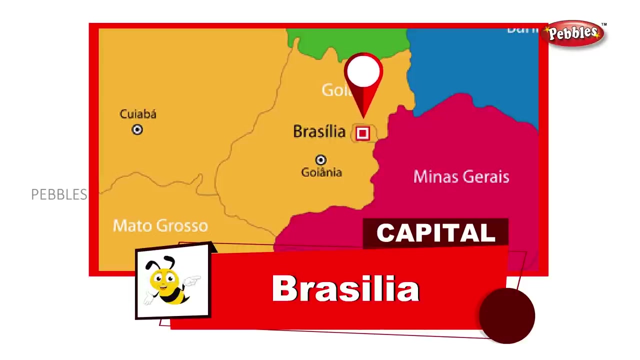 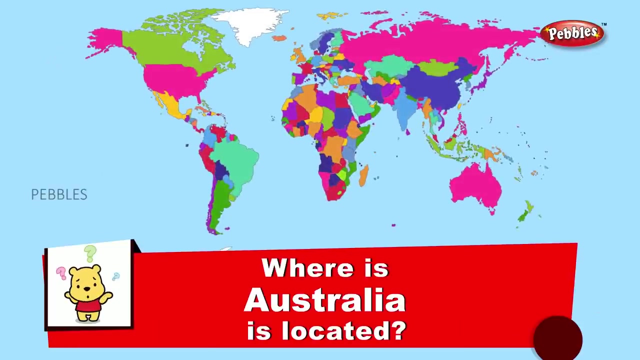 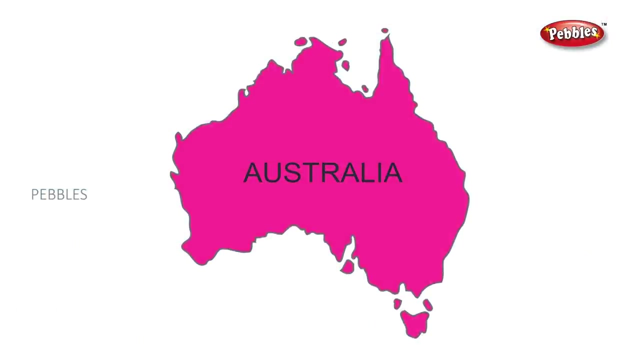 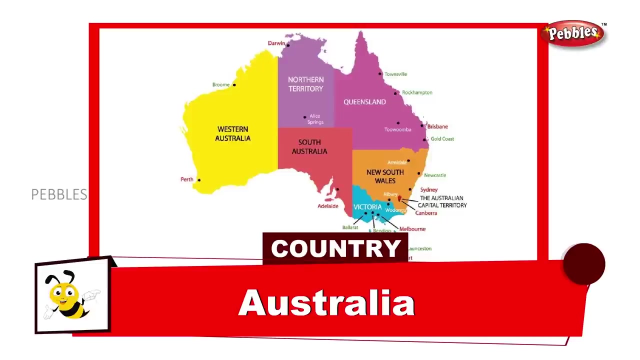 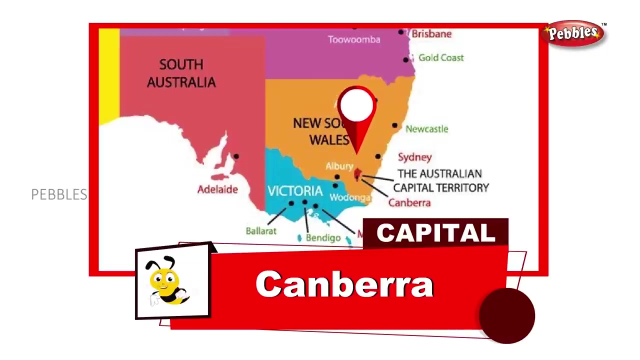 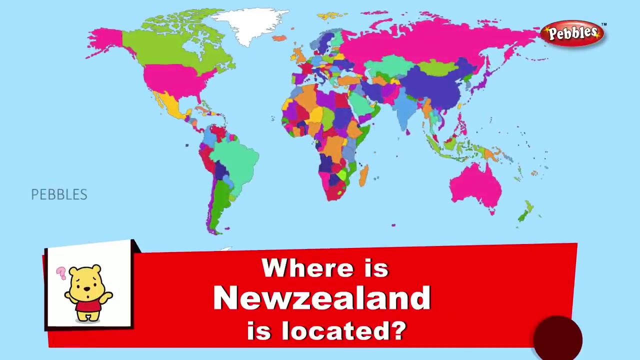 Where is Brazil located? It's here. Country Brazil, Capital, Brasilia. Where is Australia located? It's here. It's here, Country Australia Capital, Canberra. Where is New Zealand located? It's here. Where is New Zealand located.